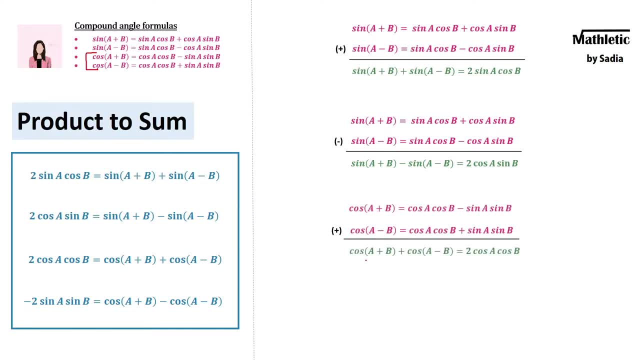 So these are the two equations. if we add them up, we get cos a plus b plus cos a minus b, as in, these two terms are added together at the left side and at the right side. these are cancelled out. you are left with cos a cos b, two cos a cos b, two cos a cos b. that's the third formula. 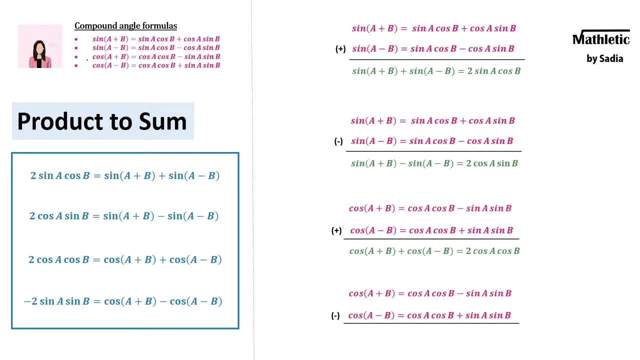 And the last one where you have to use these two formulas, but we need to use a minus sign over here. So the second equation sine will be opposite. so minus minus. So cos a plus b, minus cos a minus b. And here we have cos a- cos b minus cos a cos b. so these are cancelled out. 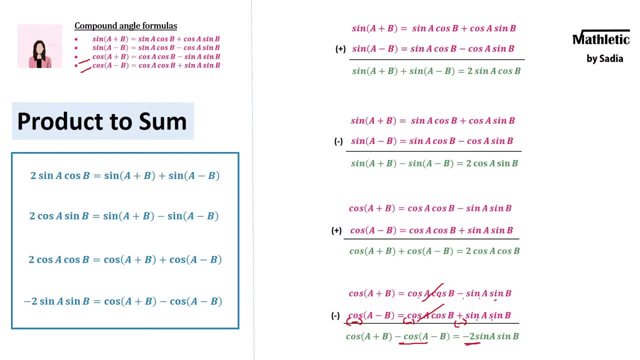 Minus sine a sine b, minus sine a sine b. so that's why minus. So this is the only formula where we have a minus. If you do not want this negative Sign here, you can shift that at the right side. in that case it will be cos a minus b. 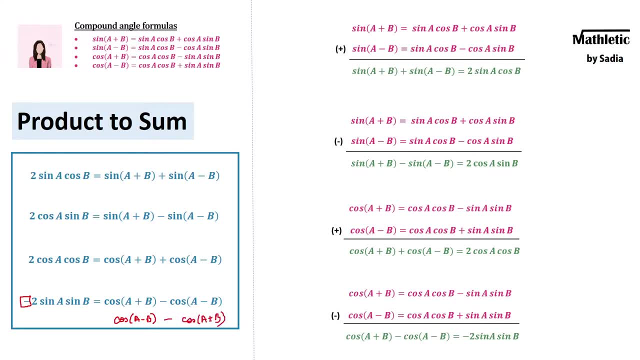 minus cos a plus b. So we are done with these four formulas. but to remember them, you can actually analyze the pattern. So whenever you are actually adding this two compound angle formulas, you will be getting the first part of the formula two sine equals b. but when you are subtracting them you will 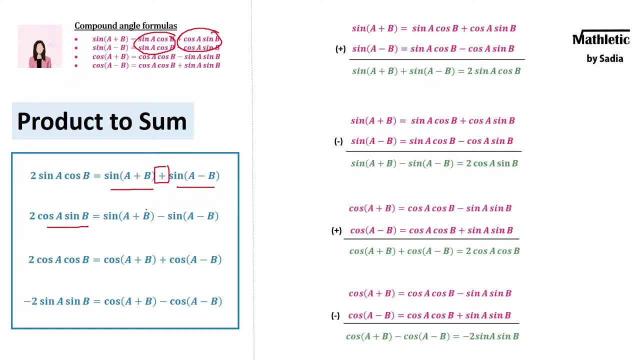 get the second part, Cos a sine b. Similarly, when you are adding cos compound angle formulas, in that case you will get the first part, cos a cos b. But when you need to deduct them, you will end up getting the second part sine a sine. 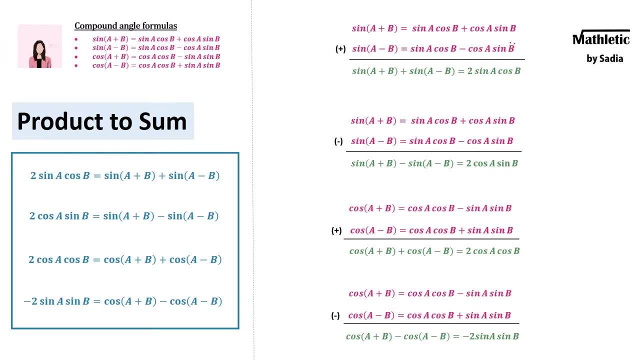 b, but with a negative sine. These four formulas are used to actually derive the product to some formula, right? You just need to write the product to some formula, right? You just need to write the product to some formula, right, You just need to change the side and that will give us the product to some version and 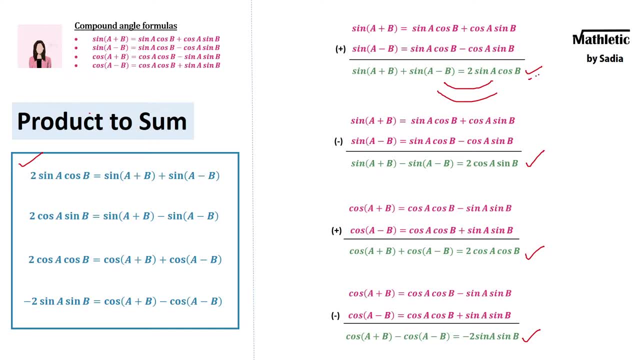 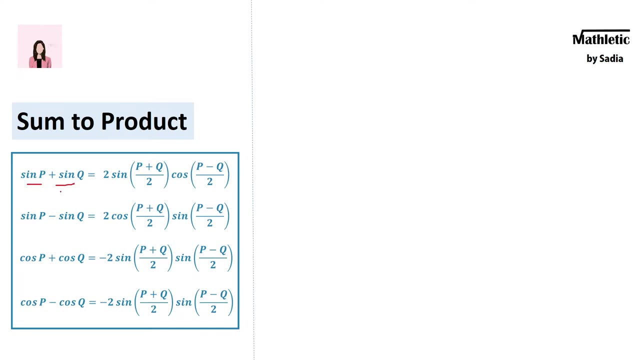 to find the sum to product, we will be using this four formulas. So if I label them as a, b, c, d, we will be using this four a, b, c, d green formulas to derive the sum to product. Sum to products. As we can see, these are added together at the left side, but at the right side it's multiplied. 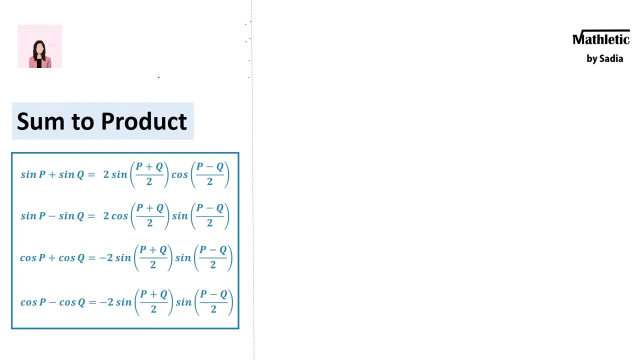 So that's why they are called sum to product. To derive the sum to product, we need to use the four formulas which I just labeled as a, b, c, d. These four formulas, If we just look at the very first two formulas here and compare them, 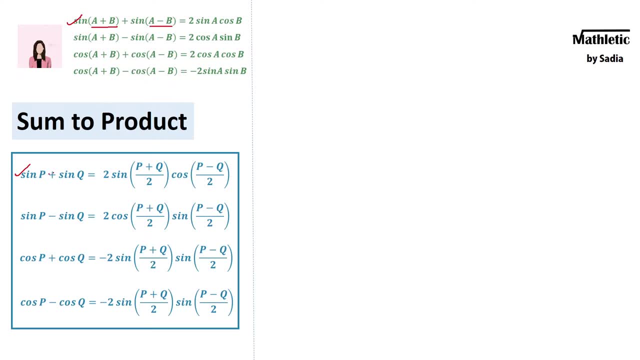 we have sine a plus b, sine a minus b, and we have sine e sine t. So the thing is, if we we replace a plus b by p and a minus b by q, In that case at the right side we need values for a and b so that we can replace them also, right? So comparing those two. 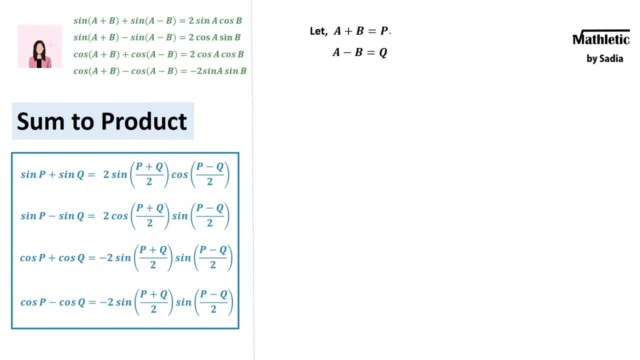 equations. we will just select a plus b as p and a minus b as q and we will solve this. two simultaneous equations Suppose this is equation 1 and 2.. We will just solve this: two simultaneous equations to get the value for a and the value for b, which we can replace. 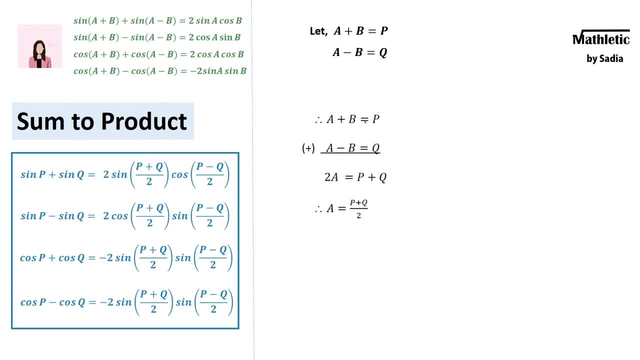 here. So equation 1, equation 2, if you add them up, this will be cancelled out. a plus a will give us 2a, p plus q. at the right side, Subjecting a will give us p plus q divided. 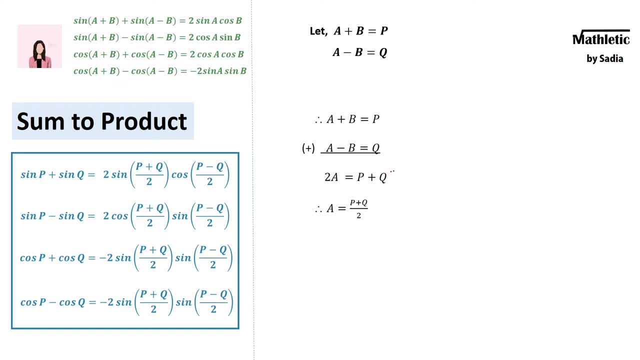 by 2.. So that's the value for a. Similarly, if we just solve this two simultaneous equations, we will get the value for a and the value for b. Use those two formulas, but instead of plus, if we use a minus, sign over here the. 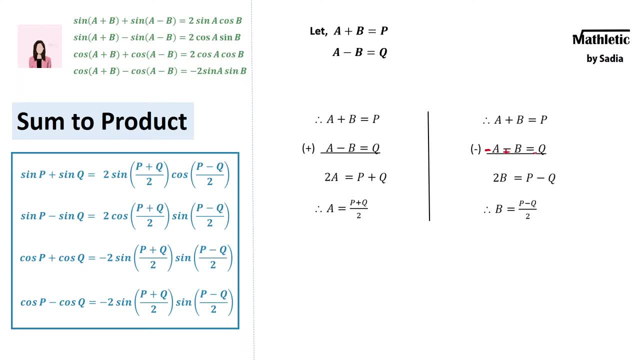 signs will be opposite: minus a and plus b, minus q. So a minus a gets cancelled out. then b plus b will give us 2b. We have p minus q at the right side, So subjecting b from this equation will give us p minus q divided by 2.. So this is the value for a and b. So 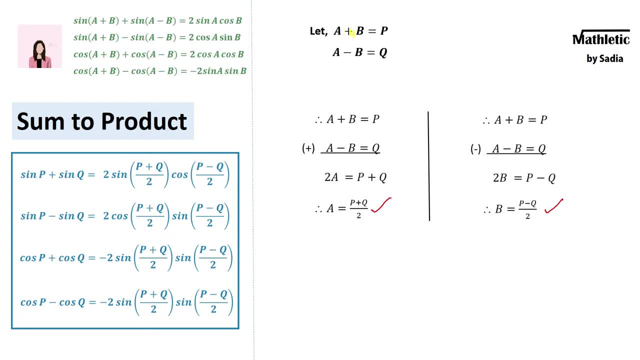 now we have. We have four values, as in: a plus b is p, a minus b is q. Then we have the value for a, we have the value for b. All these four values need to be replaced here, So this: